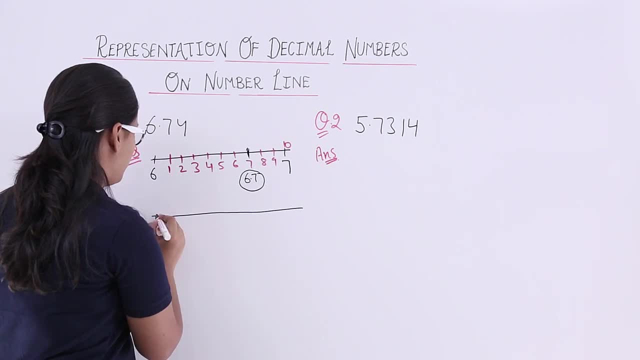 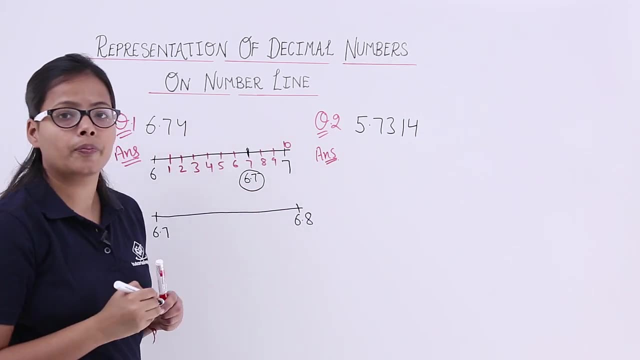 number 3, 5 and here number 7.. Now again, you need to a number to draw this. So you need to draw 6, from 0 to 8, as here. AND here number 3 I have drawn because You can see that I haveanhcleim and I have. 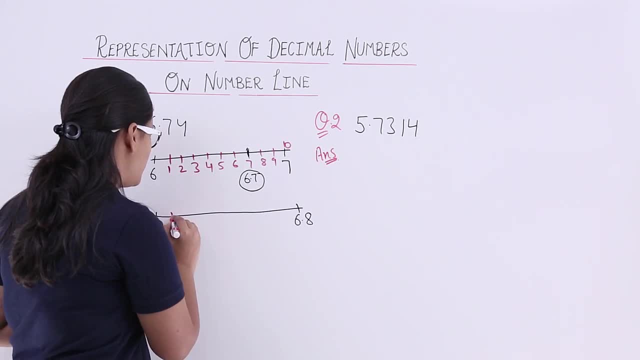 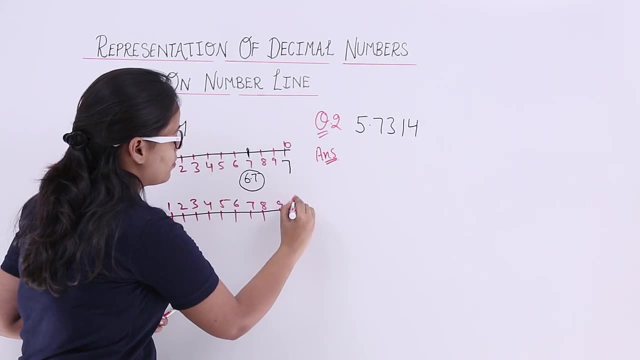 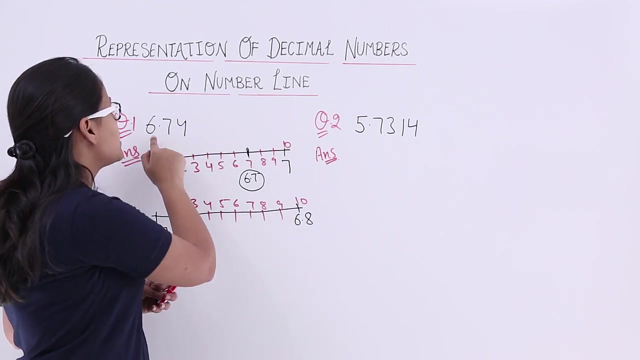 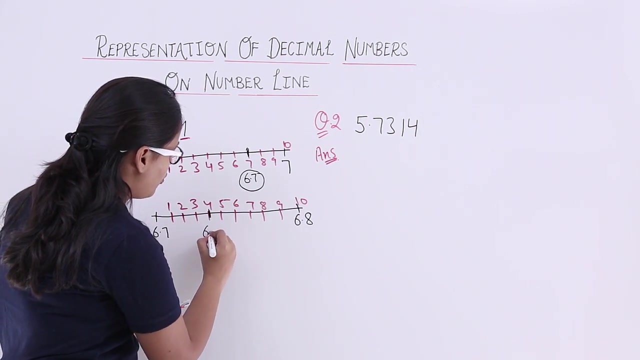 What you will do again. You will again segment this into 10 parts, and this 10 is 6.8. and now what you need to relocate here You need to locate 6.74.. As you can see here, the second decimal digit is 4.. So where will be the point? You can see here, it is 4. 6.74.. To have the 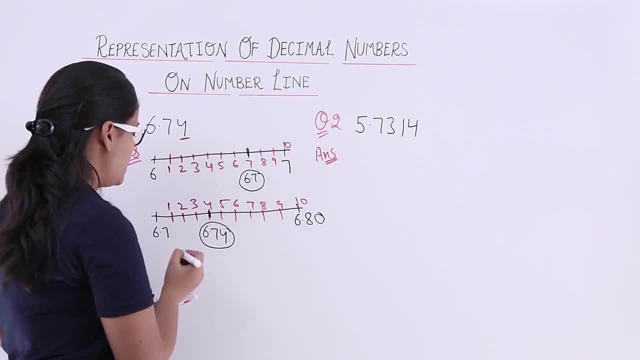 clear understanding what you can do, Write 0s here: 6.0, 7.0.. So that you can understand that these are the decimal digits: 0.1, 0.2, 0.3, 0.4, 0.5, 0.6, 0.7, 0.8, 0.9, 0.9, 0.10,. 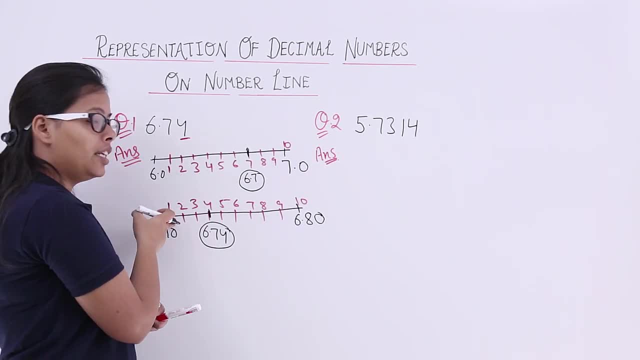 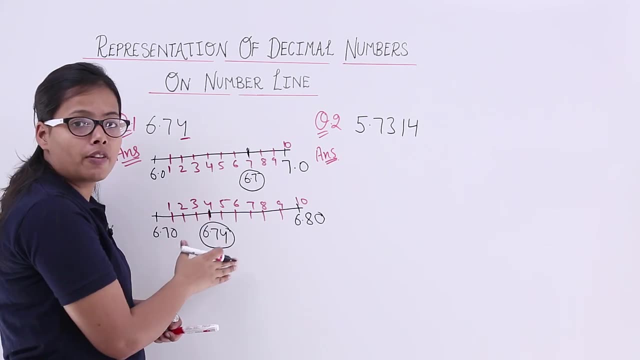 0.2, 0.3.. Here these are the decimal digits: 0.71,, 0.72,, 0.73, 0.74, up to so on. That's why 6.74 is lying here on this second number line. I hope you understood this question. 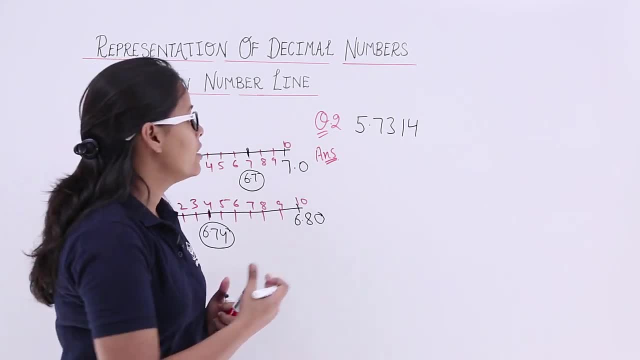 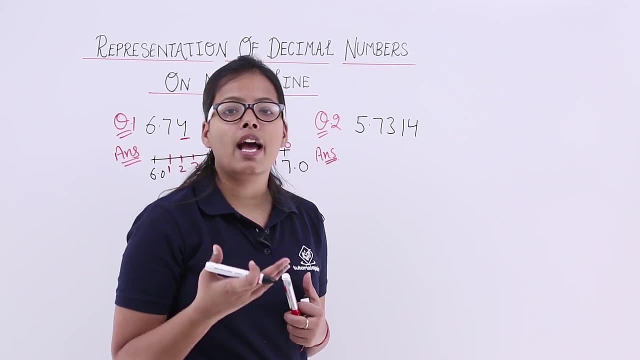 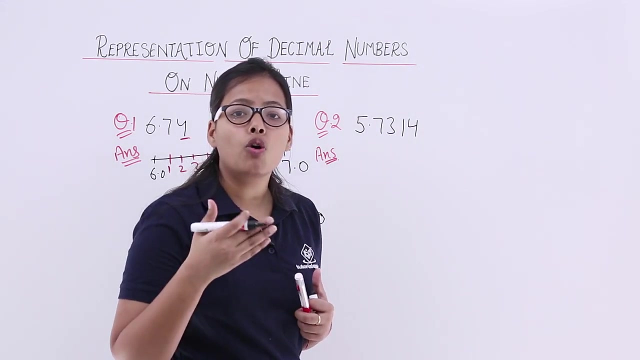 quite well, Now let's take our second question, which says 5.7314.. What you will do? You saw in the previous example that I have followed two steps, As here you can see there are 4 decimal digits, So I will follow 4 steps to plot the final. 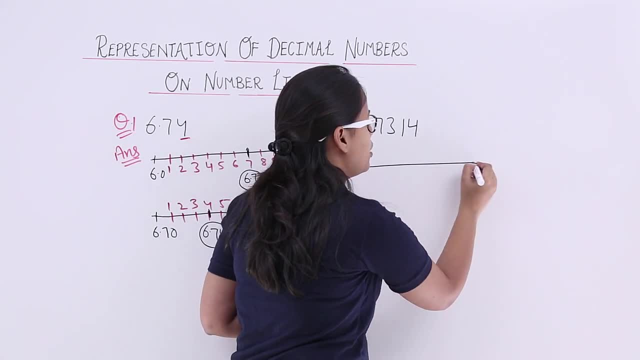 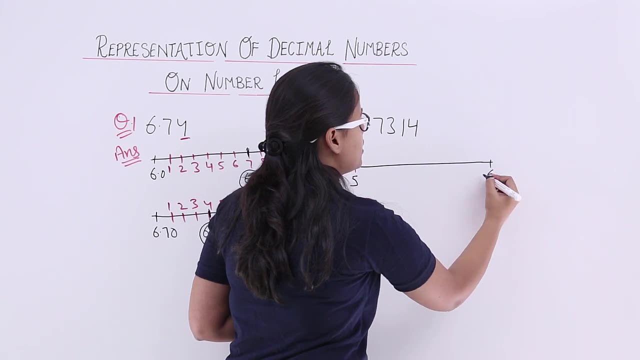 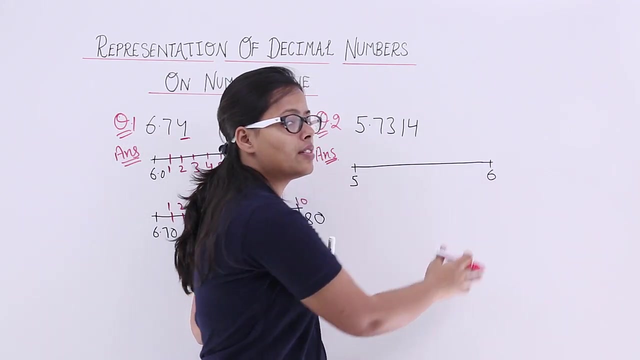 result. So let's start with our first step: Plot 5 and 6.. As this number is greater than 5 and lesser than 6.. So I have plotted 5 and 6.. Now what you will do, You will segment. 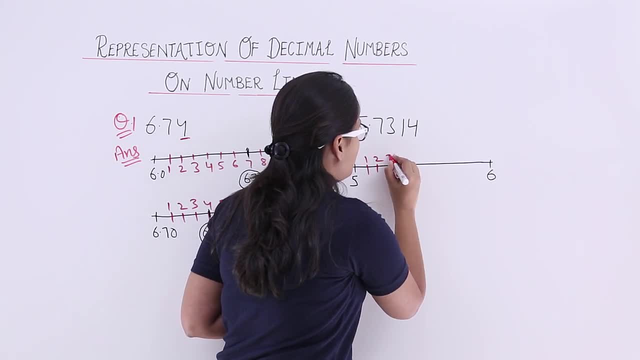 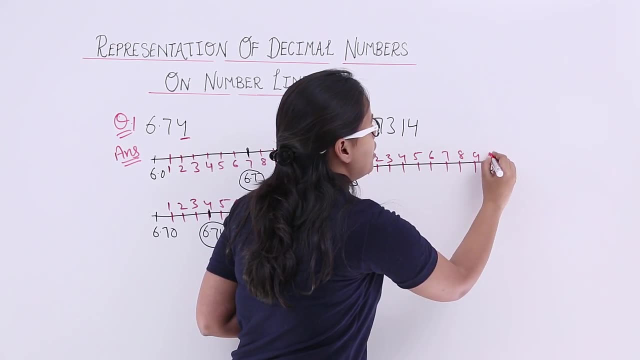 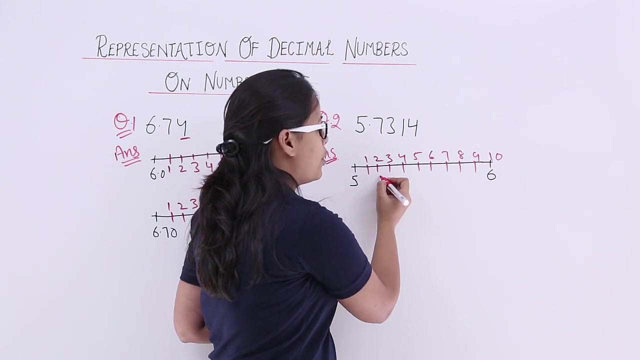 this: 1,, 2.. 3,, 4,, 5,, 6,, 7,, 8,, 9 and 10.. These are the decimal points between 5 and 6.. This is 5.1,. 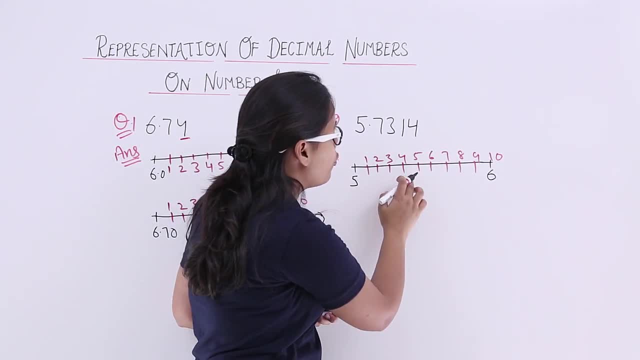 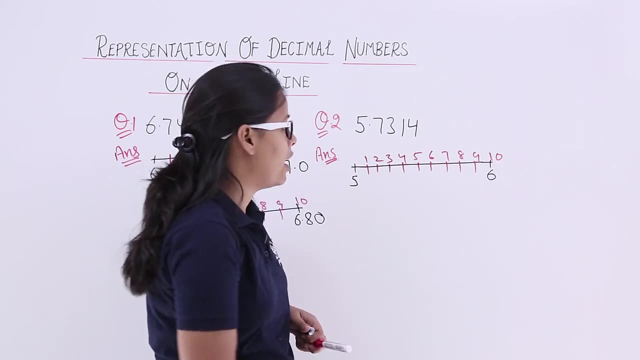 this is 5.2,, this is 5.3,, 4,, 5 and so on to 6.. What you need to plot, You need to plot 5.7. and where is 7?? You can see, 7 is here. 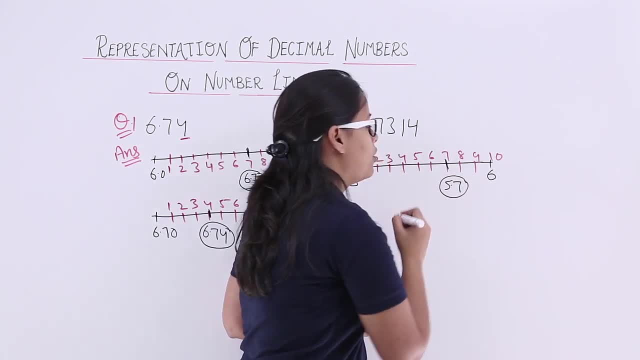 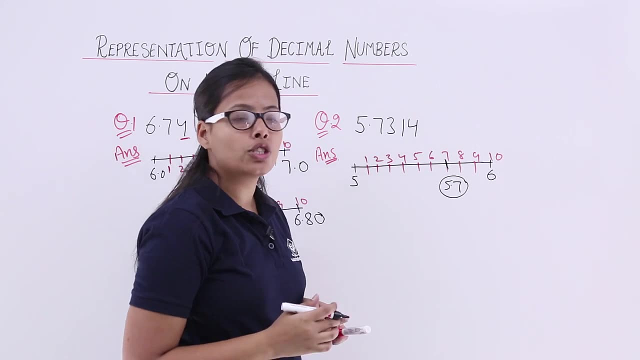 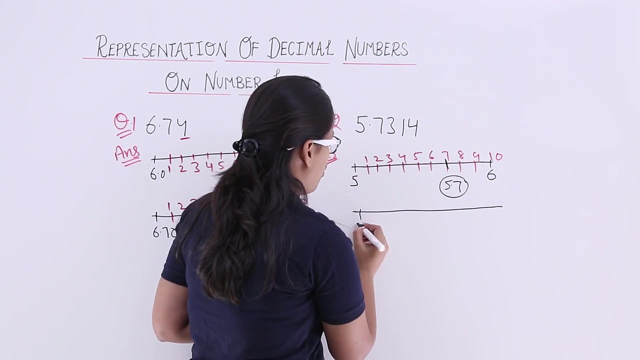 7,, 2 and 7.. So what will be the answer? 5.7 on the first number line. Now you needmark 1.. 2 and 2 are equal to 10.. You will plot see that. so 4, 4,, 5,, 6,, 7,, 8 and 10.. This is 5.3.. So what you will do, You will again take a number line and draw 5.7 here and 5.8 here. So what you will do, You will segment this again into 10 perspective, You will again draw this number, It will be 15asu, and then, if we will take aencia in, .5 is 1诊 at the next. 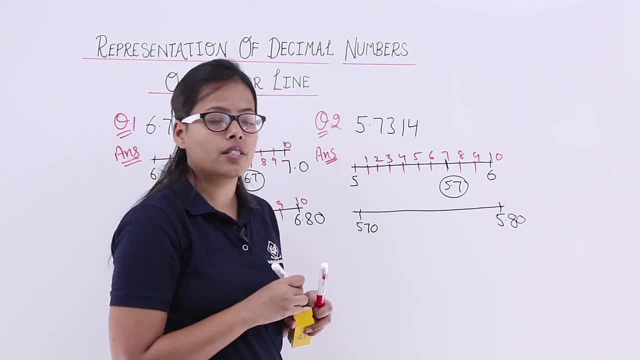 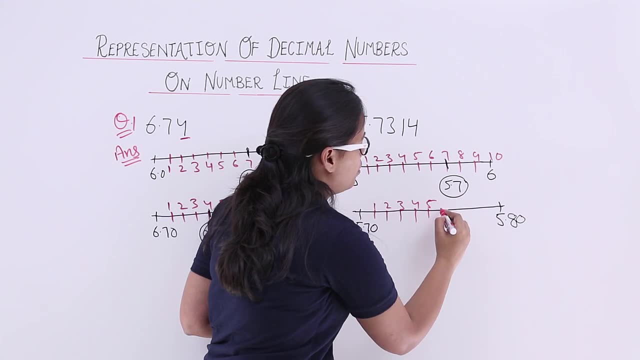 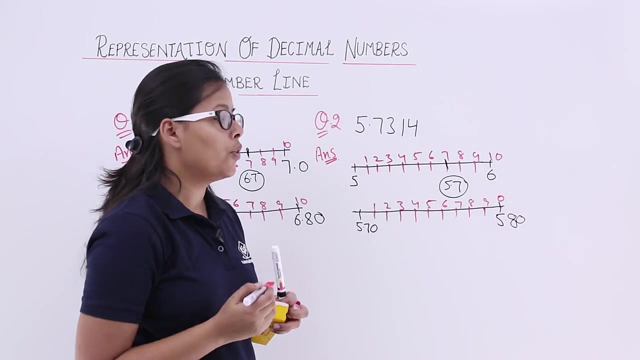 number at the right. So the number line must add 5 and then, additionally, will add 2s to this column. All numbers will be added on the number line. So what will be the answer? 5.7 on the number into 10 parts: 1, 2, 3, 4.. This will go on up to 5.80.. What you need to do now You need. 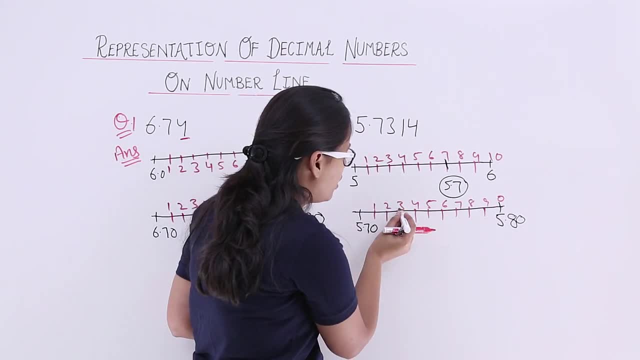 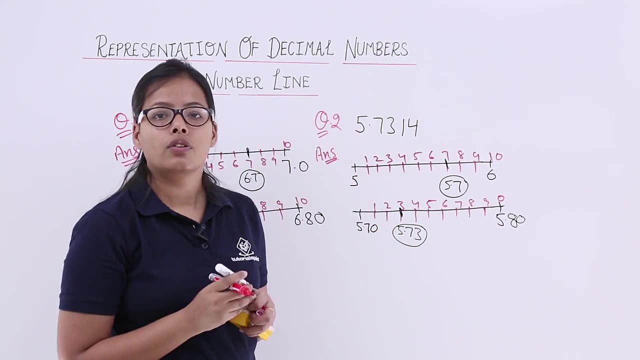 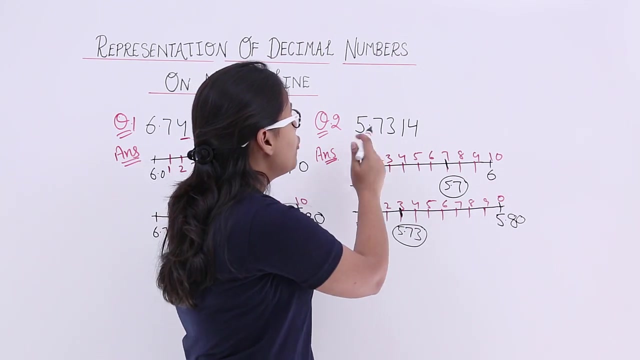 to plot 5.73.. You can see here, here is 3.. So this will be the final result for the second decimal point. Now what you have to do? You have to plot 5.731 on a number line. So what? 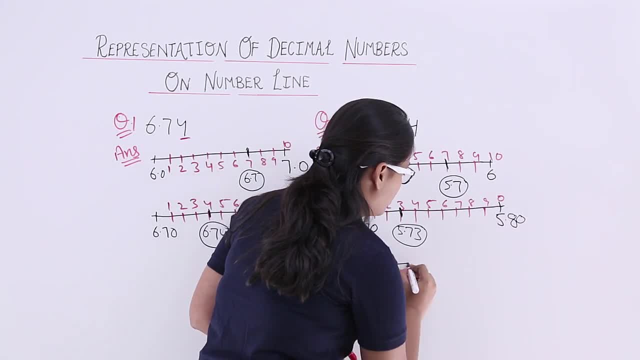 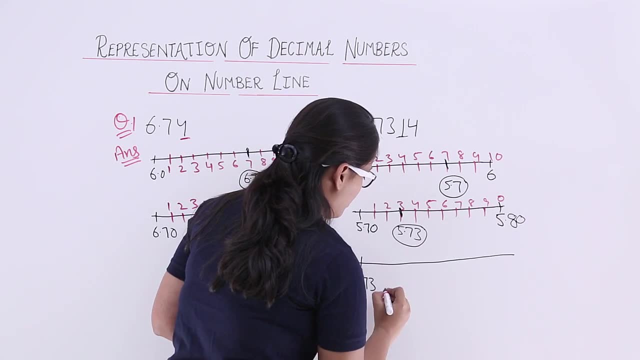 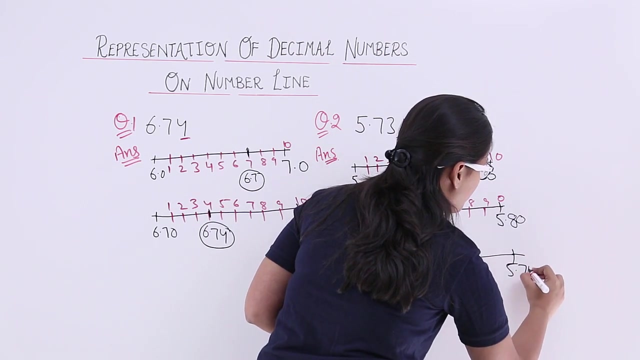 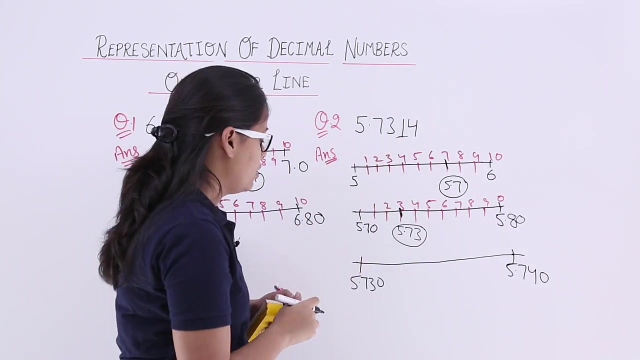 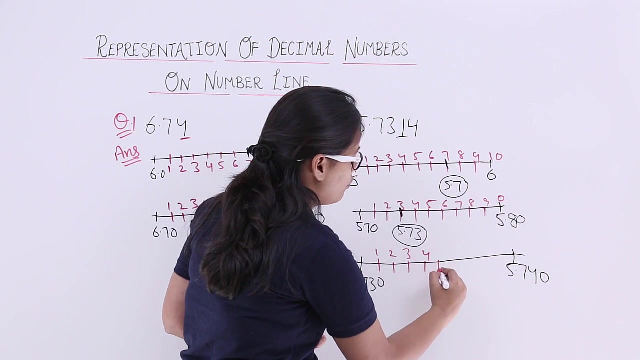 you will do? You will plot this line, third number, line 5.730, up to 5.740.. What you need to plot here? You need to plot 1.. So what you will do, You will segment this: 1,, 2,, 3,, 4,, 5,, 6, and this will go on to 5.730.. So this will 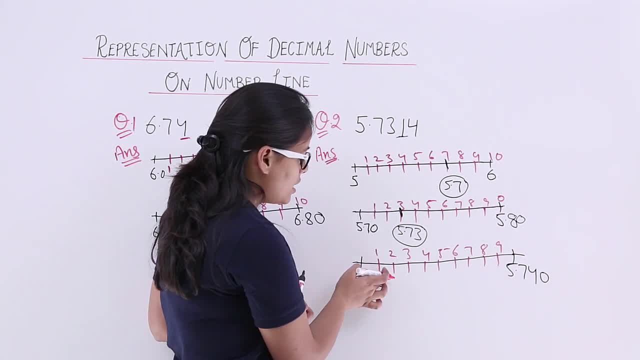